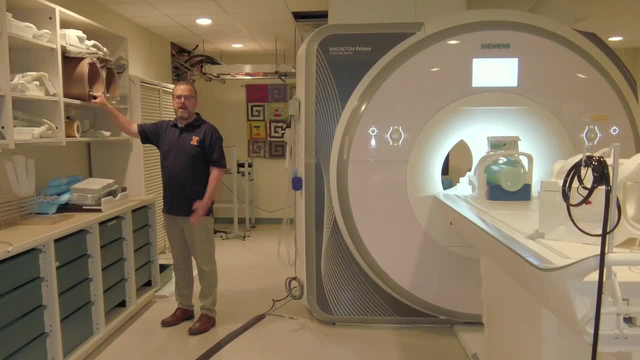 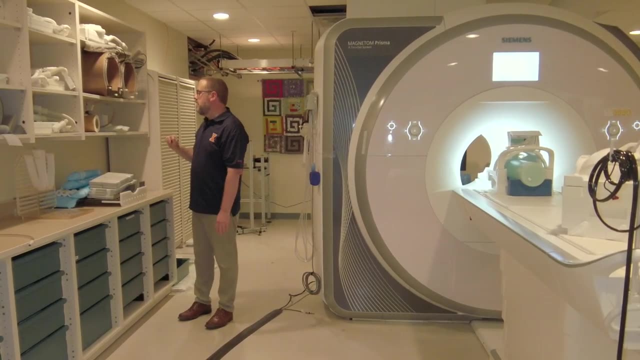 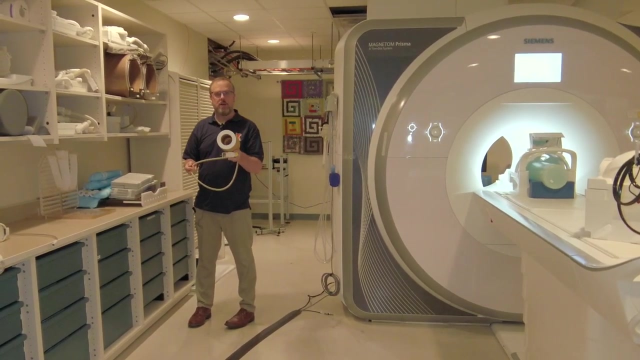 Sodium is really important for neural tissues. You have sodium and potassium are the two chemicals that really create the membrane potentials, And so sodium is really important. And then we also have other coils that can accommodate a variety of other things. So this right here is a small animal. 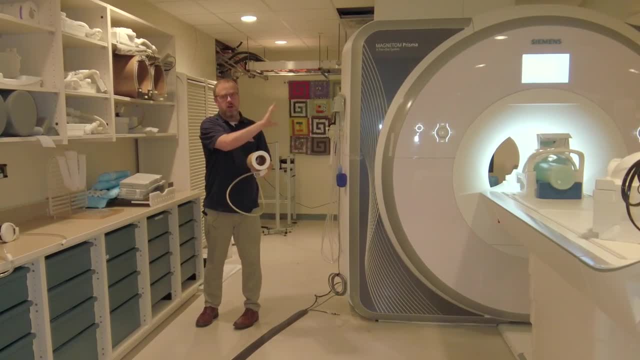 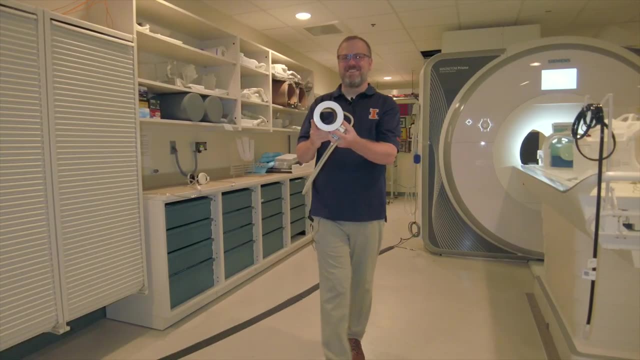 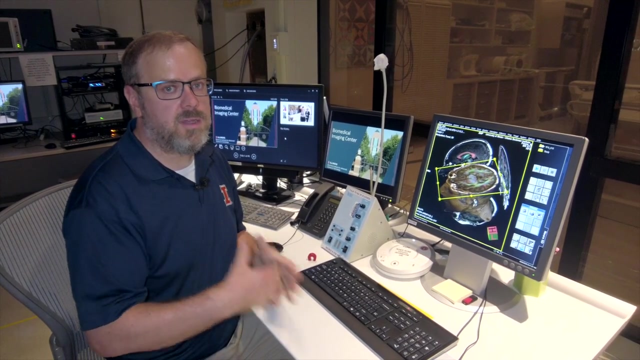 coil So you can put a small animal in here and you can still, even though it's a really large bore MRI system, you can image things fairly small, such as a rat, a mouse or an octopus. One example of things that we've done here over a long time is exercise studies in older adults. So we take 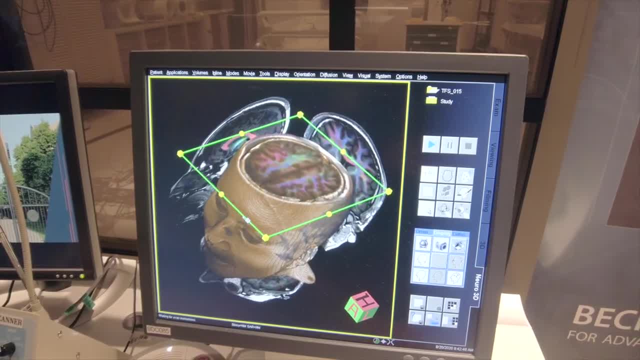 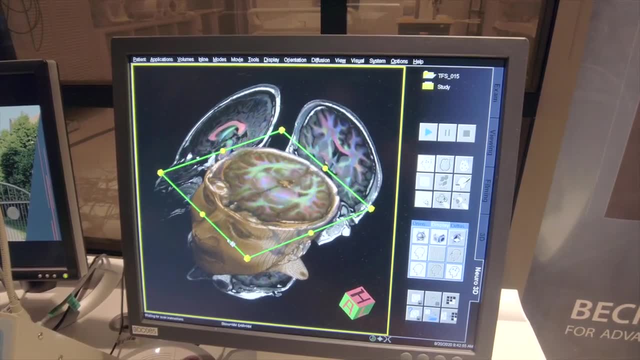 older adults who are relatively sedentary, and we put them on aerobic fitness program And in just as little as a couple of months we can actually see changes in the structure of their brain that come from that improved health and cardiovascular fitness And that lets their brain work better. 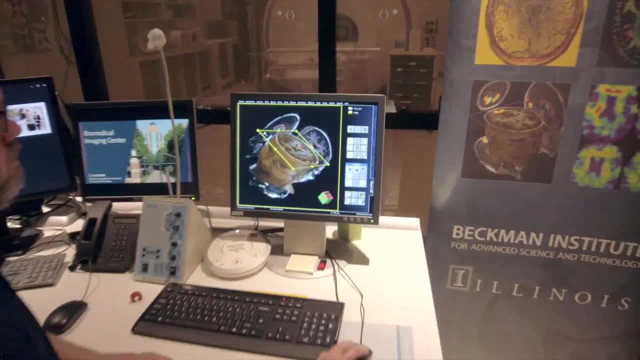 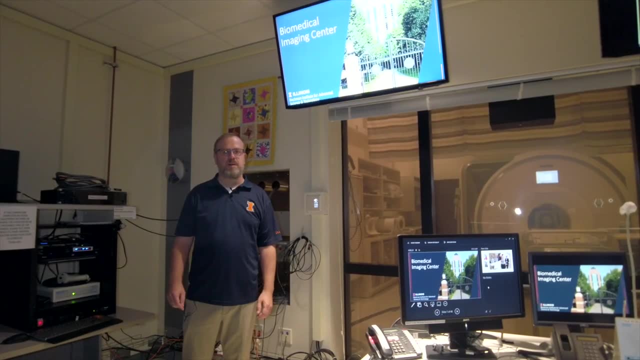 We can give them tests. They do better on the tests and we can see their brain and see the representation in their brain about the structures that actually change. to support that, In addition, we have a number of unique acquisitions that I wanted to tell you about that are very unique to 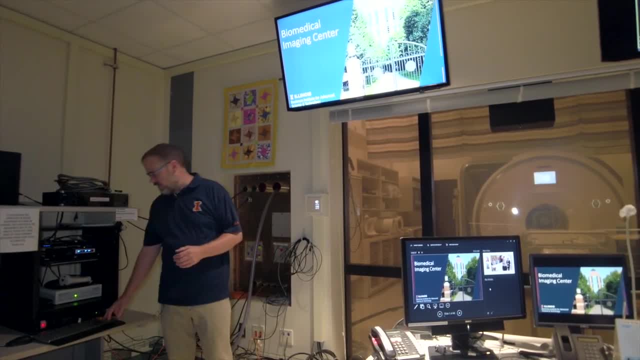 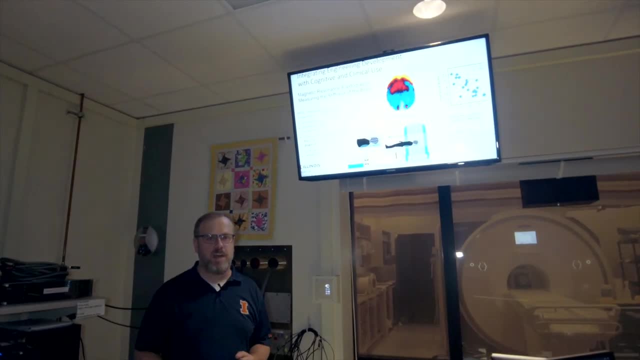 the Biomedical Imaging Center here that we're applying in a wide range of circumstances. The first of those is magnetic resonance elastography. What we do is we put a little vibration pad behind the head, We gently vibrate the head and we watch to see how the brain tissue moves. and we can. 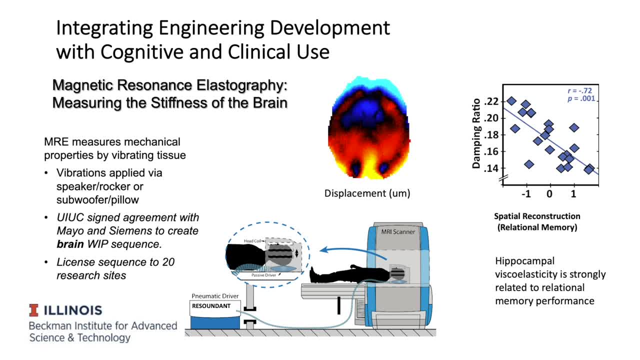 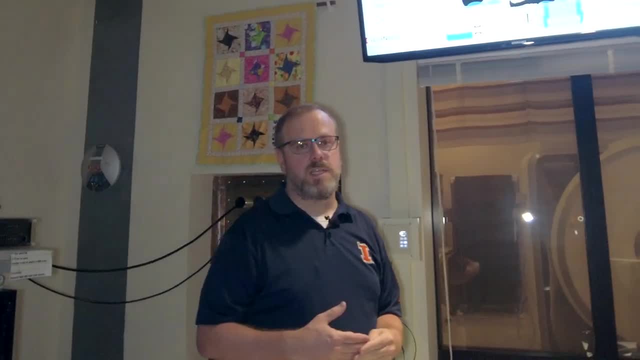 estimate the stiffness of the tissue. We show sort of the general process here, where we have a resounded device and we have a pillow placed behind the head and we can acquire really high resolution brain images. So what's unique to here is we have a very customized 3D multiband sequence that we use. 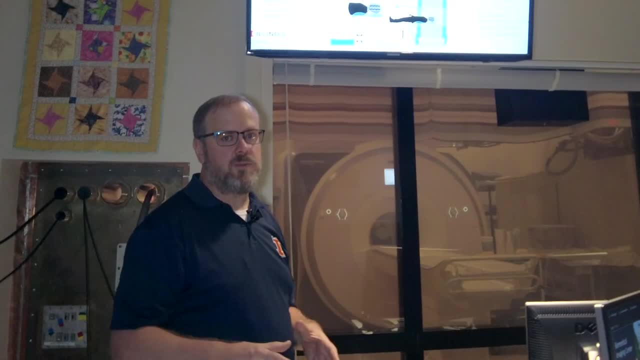 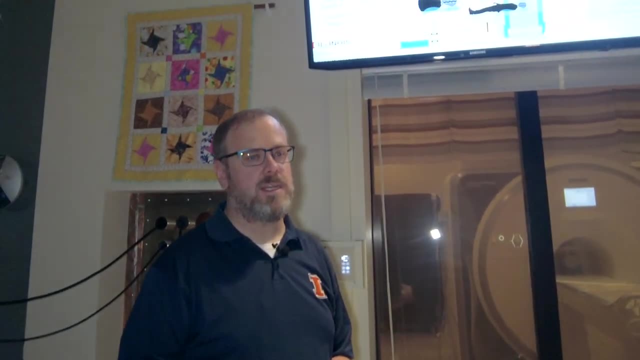 that has some spiral acquisition, that gives us a really good signal-to-noise ratio to provide high resolution, high signal-to-noise ratio for being able to get really good, high quality mechanical property maps of the brain. And so one of the exciting results we've had is in healthy college. 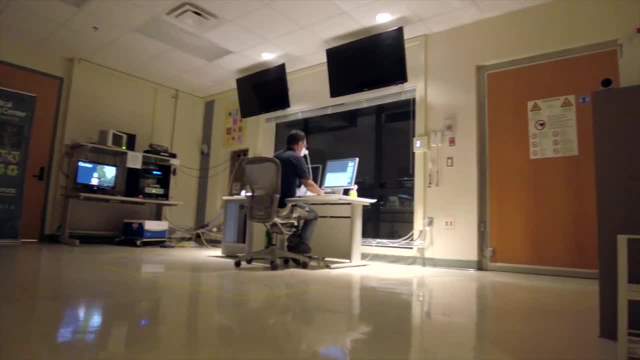 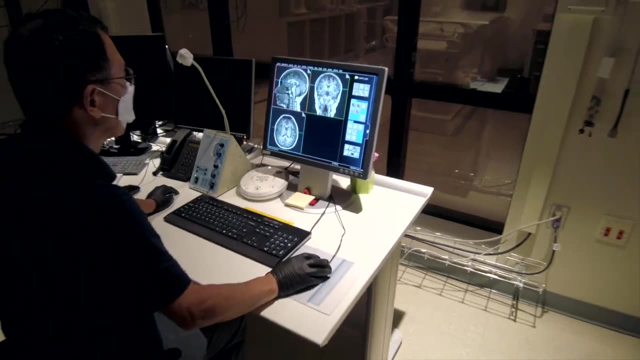 age kids. we're able to find a measure, which is the damping ratio of the hippocampus, that correlates with their memory performance. with a really high correlation coefficient, We're explaining about 50% of the variance on their performance, So we're really excited by that. 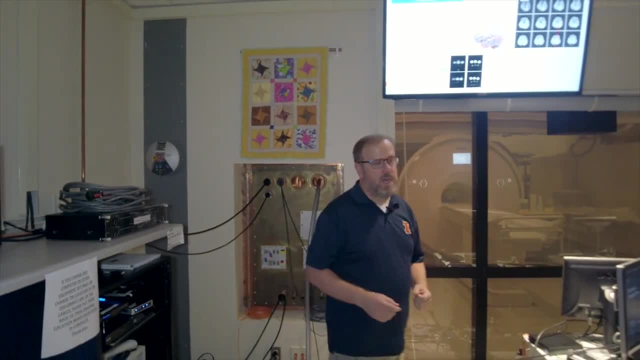 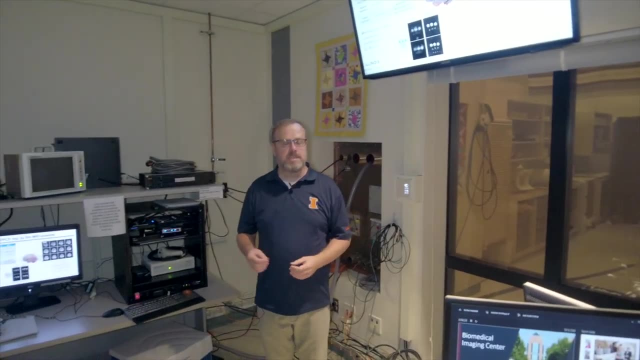 The other acquisition that we have here that's unique to here, is a spectroscopic imaging acquisition, And this is the work of Professor Liang in electrical and computer engineering department, And what he has done is he has developed a sequence that can provide 3D high. 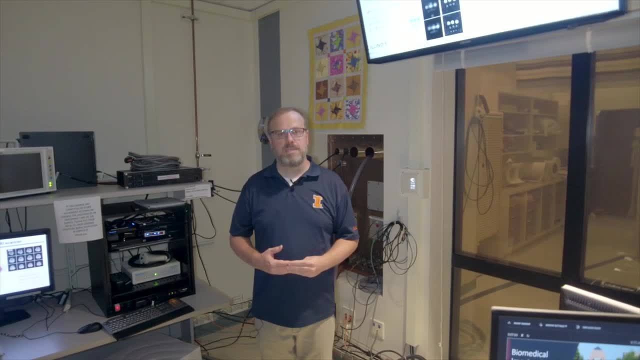 resolution: chemical information about the brain. So you can see many of the metabolites that are active, And so we show an example of that here. We can take the brain. We can break it up into lots of different chemicals. Each one of these. 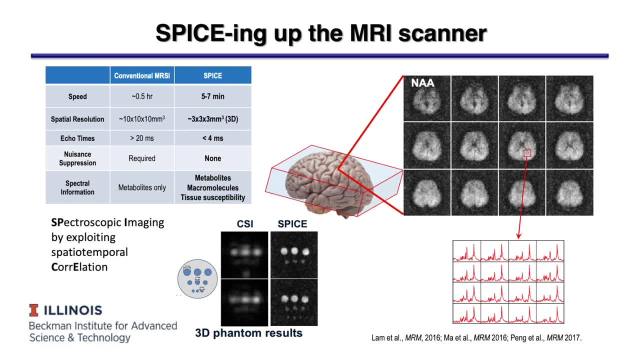 The spectra give us information about the different chemicals that are present, So we can pull one out. We pulled out NAA, which is a marker of healthy brain tissue, But we can make a map for about nine or 10 different chemicals in the brain associated with that. What makes 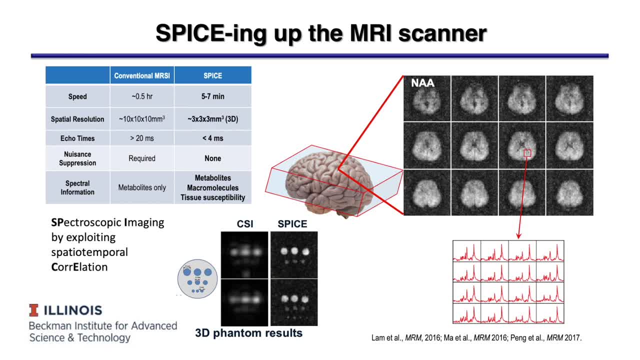 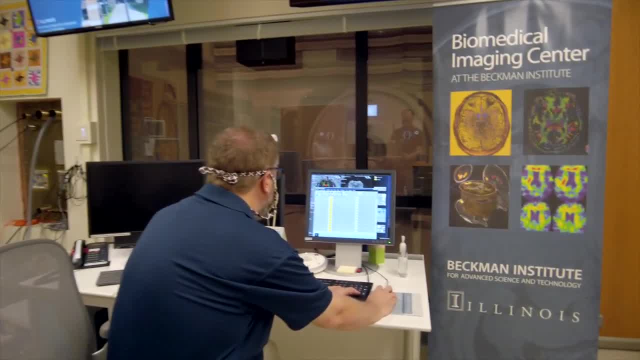 it unique here is we can get all of this, in addition to myelin information, resting state, functional connectivity, lipid content, all in under 10 minutes, with a 3D scan of the brain at about two to three millimeter spatial resolution, And, as you can see too, we have a lot of. 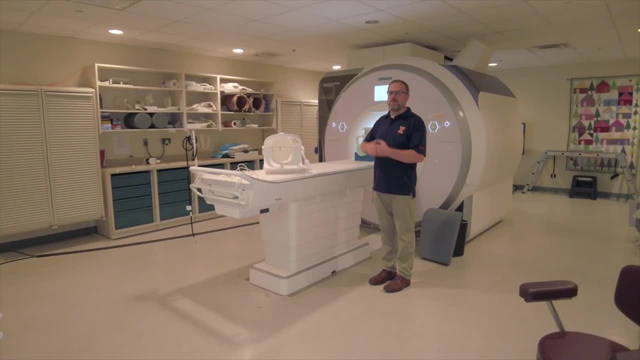 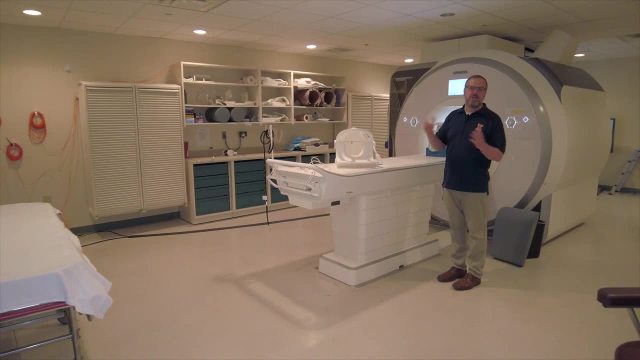 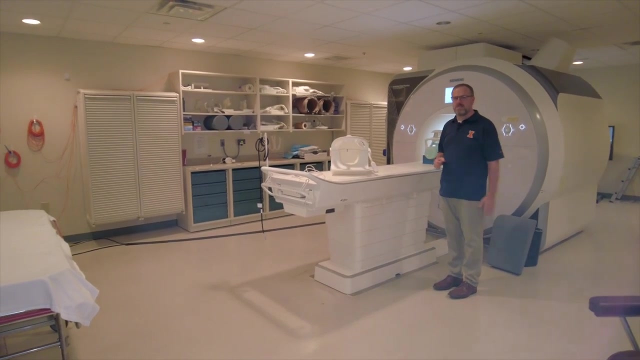 space in this room in order to do experiments. So we have people doing EEG electrodes, eye tracking, functional MRI paradigms, And then we're even having new users coming from, say, aerospace engineering to do fluid flows and the like. So lots of flexible space in order to be able to. do the experiments. 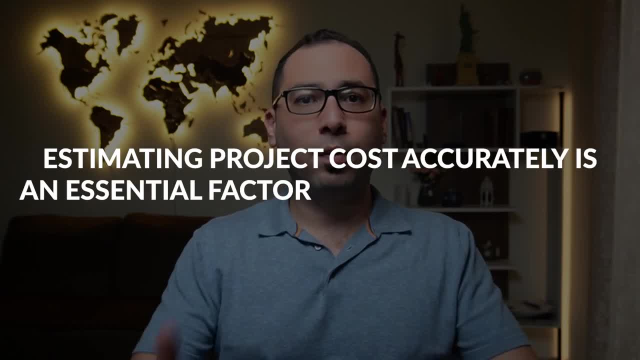 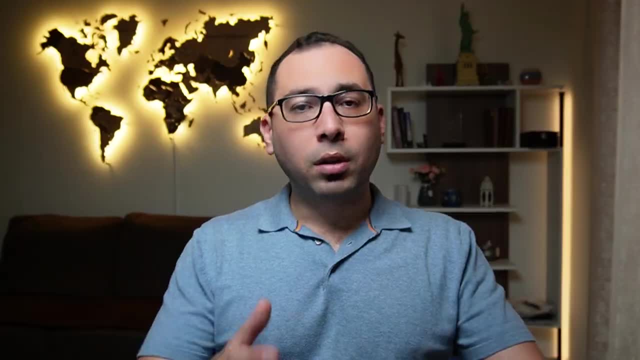 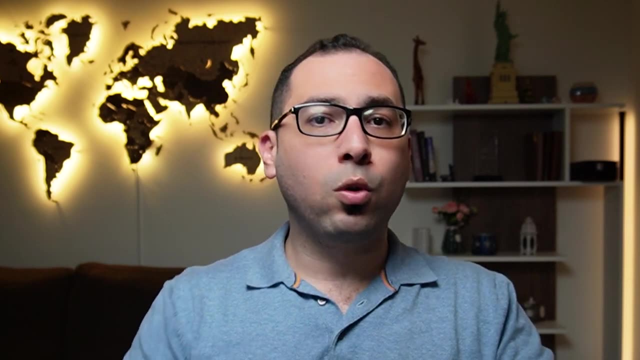 Estimating project cost accurately is an essential factor for project success. That's why, in this video, I'll walk you through project cost estimation and why it is called estimation. Also, what are the cost estimating methodologies that we usually use to estimate the cost of projects? And, if you stay until the end of the video, I'll share with you some numerical 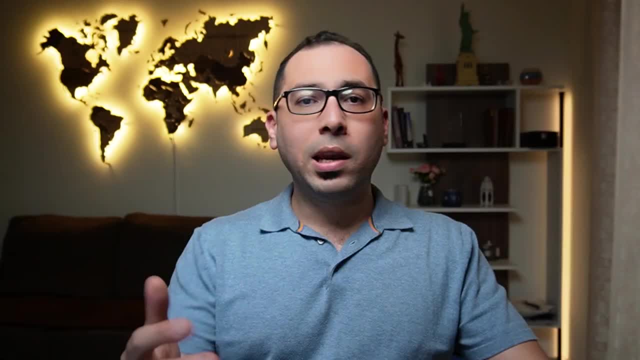 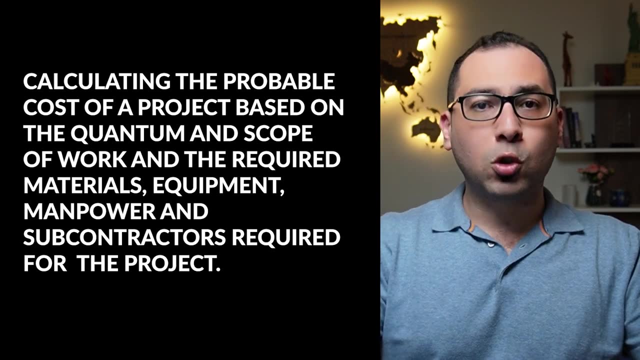 cost estimation examples for you to understand how it works. And let's begin with. what is cost estimation? Cost estimation is calculating the probable cost of a project based on the quantum and the scope of work and the required materials, equipment, manpower and subcontractors required. 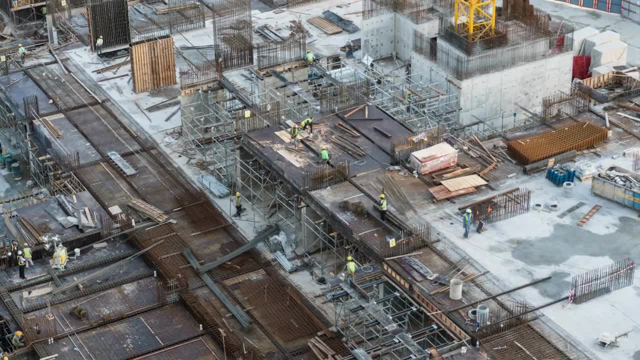 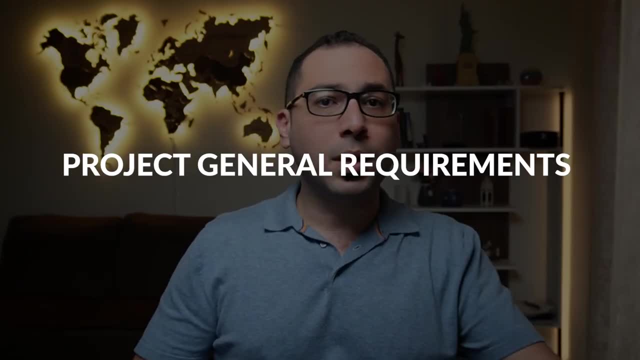 Also, in construction sites, there is a huge amount of uncertainty because so much of the material that you are using is not coming from the project. works are there and so many parties are involved in the construction, Not forgetting to mention project general requirements and material wastage and so on.